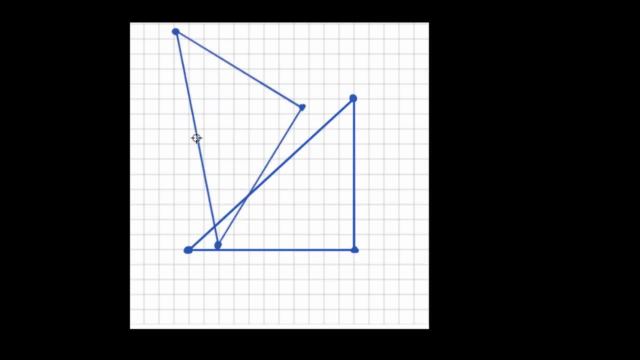 That is a dilation, Or I could scale it up: This is also a dilation, or even going off of the graph paper. So the whole point here is just to appreciate that we don't just have the rigid transformations, We can have other types of transformations. 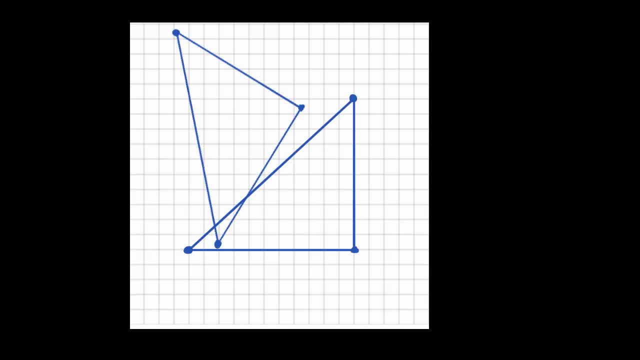 And dilation is one of them in your toolkit that you'll often see, especially when you get introduced to the idea of transformation. 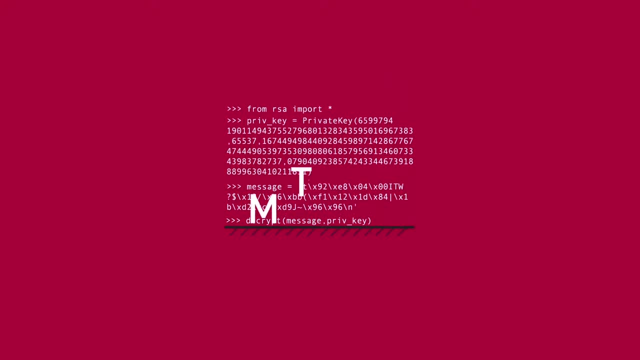 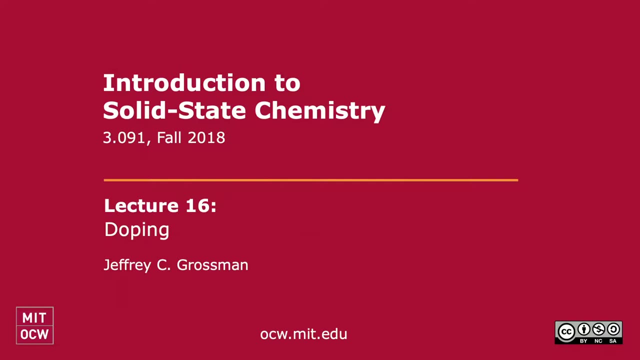 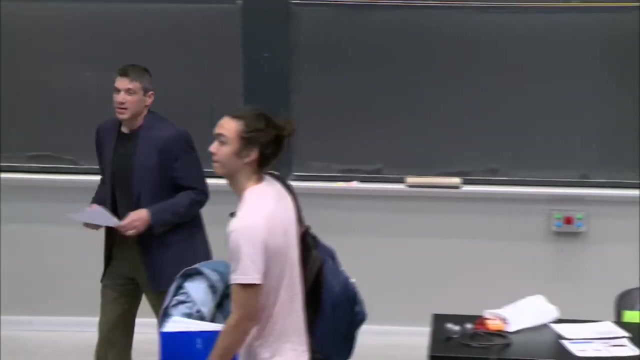 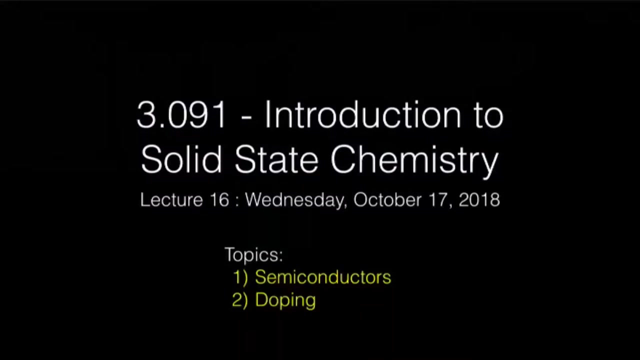 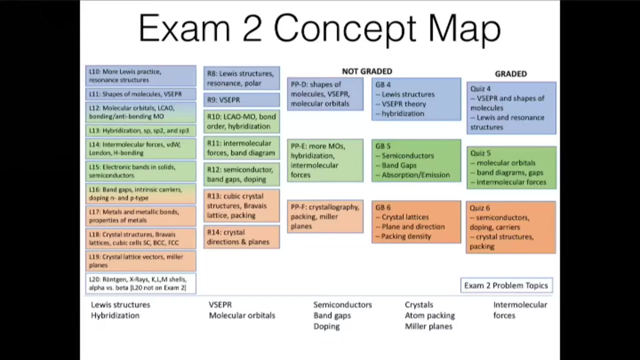 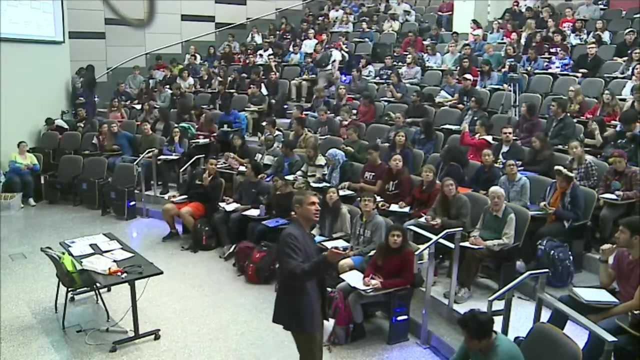 We are talking about semiconductors today. Yeah, yeah, yeah, And I finished our exam to concept map that I thought maybe you guys would find useful. This is much like the last time when I gave you guys the concept map. I'm just giving it a little earlier this time And here you can. 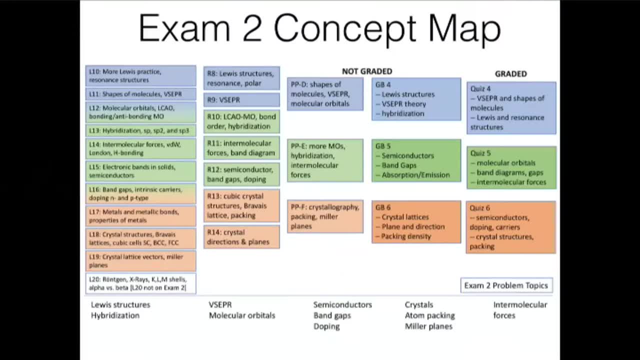 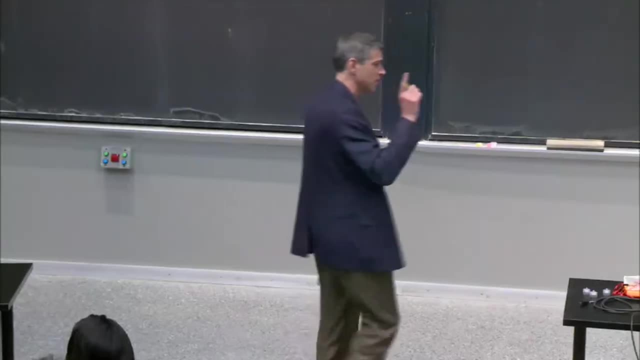 see all the connections right between the lectures, the recitations, the problem sets- okay, the quizzes and the quizzes over here, the goodie bags and the exam topics. And speaking of the quizzes, tomorrow there's a quiz And so you could look up here and say: 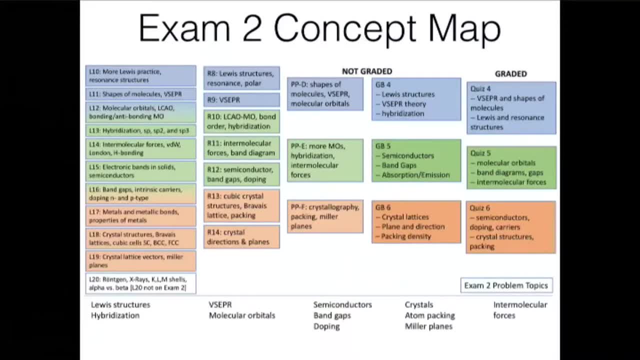 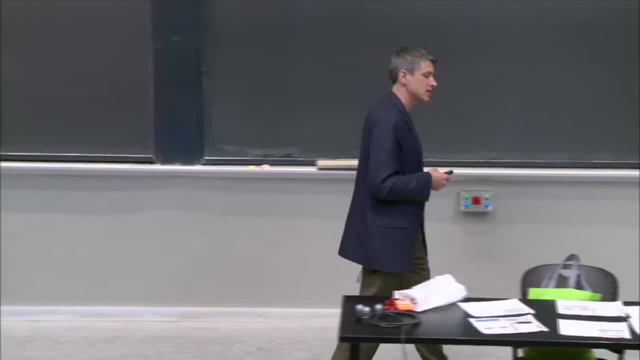 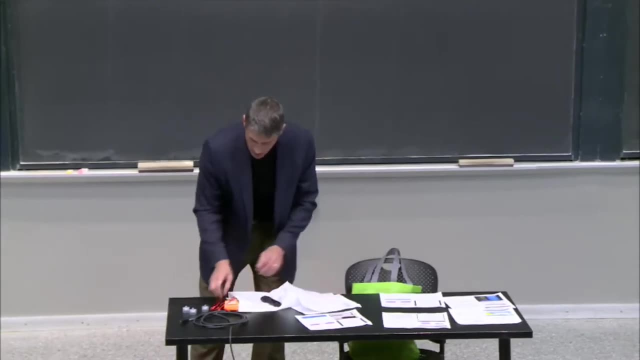 okay. well, what's going to be on that quiz? right? Might cover some molecular orbital theory. might cover the bandgap stuff that we did on Monday and that you covered in recitation yesterday. Oh, and your intermolecular forces we also did And you're asked to bring to the quiz. 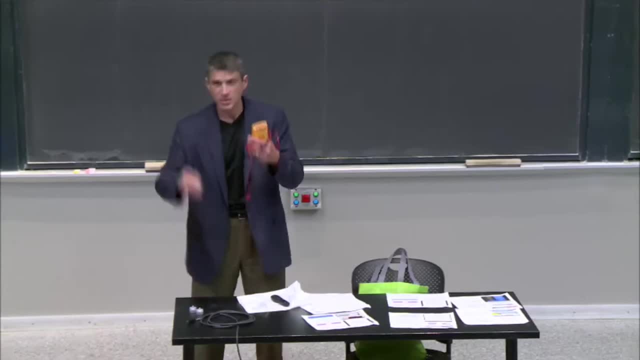 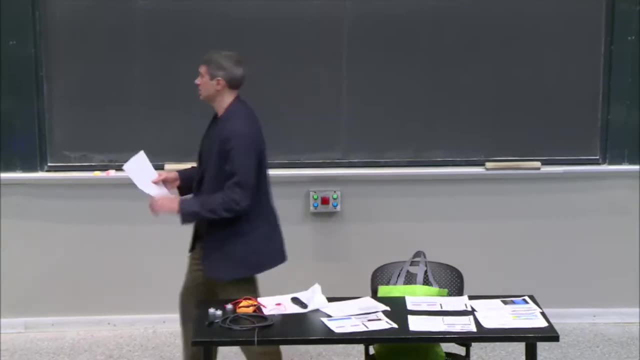 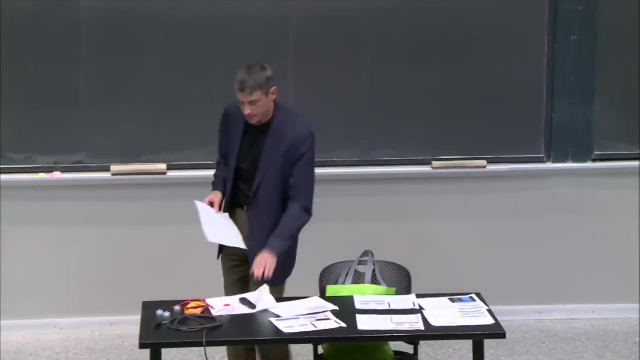 the voltmeter and these large LEDs. okay, Now I'll talk about that a little bit more about this in a few minutes. okay, So remember to bring that. Laura will also send a reminder email about that. Okay, you have voltmeters, You have?